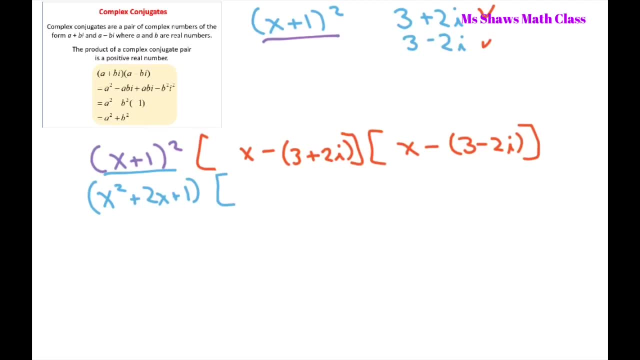 just your factoring facts, And here I'm going to move the parentheses around. So I'm going to write this as x minus 3 plus 2i, Alright, And the same thing here: x minus 3 minus 2i. So it's just a little trick and this is: 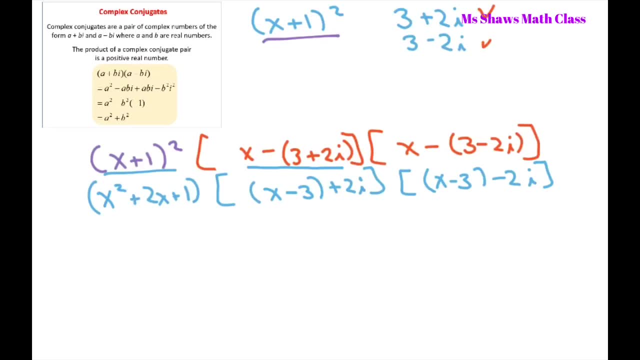 going to help us get rid of the i's before we start combining all these terms And condensing this. So basically, what I did is I wrote this as a plus bi, that's what we have here, and this going to be times a minus bi. In this case, our a is x minus 3 and our b is 2.. And then 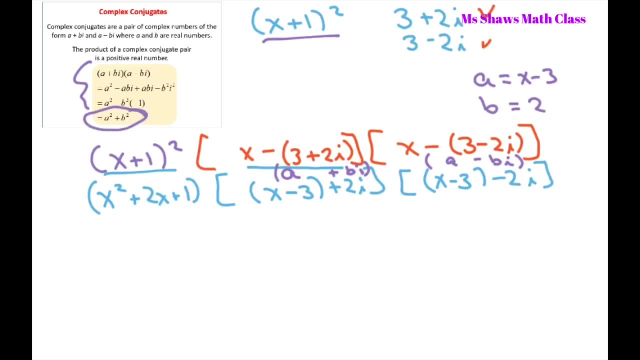 I'm just going to follow this here and use the fact that a plus bi times a minus bi equals a squared plus b squared. So let's write that out: x squared plus 2x plus 1.. Again, this is our polynomial p of x. Alright, and then? so my a is going to be x minus 3 and you square. 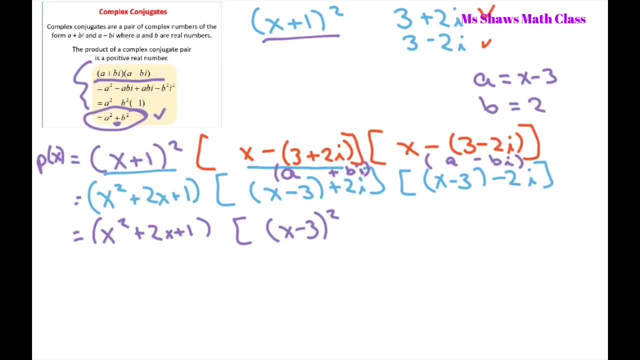 it. Then you put the plus plus your b, 2 squared, So that gives us x plus – I don't know- squared plus 2x plus 1.. And this part right here is just x squared minus 6x plus. 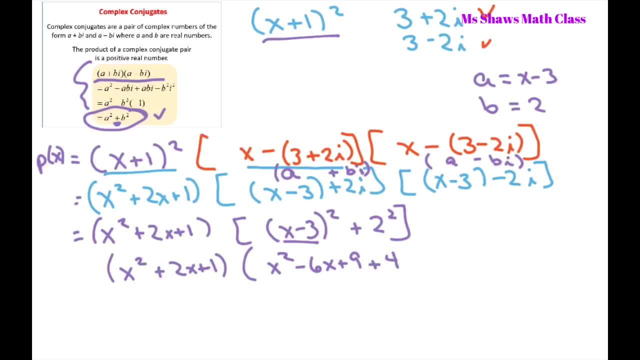 9.. Then you have the plus 4. And this equals 13.. So finally, we have x squared plus 2x plus 1 times x squared minus 6x plus 13.. Now, if you were given this to factor on a test, it. 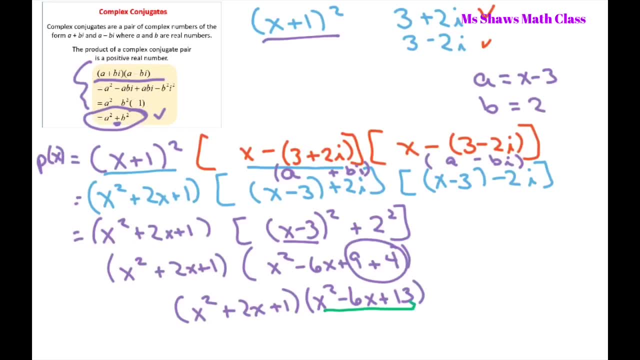 would have to use a quadratic formula And when you used it, you would get these two zeros, complex zeros. Now, to form our polynomial, you're going to have to, you know, combine all these terms, like FOIL this out, And you're going to get nine terms. It's very boring.